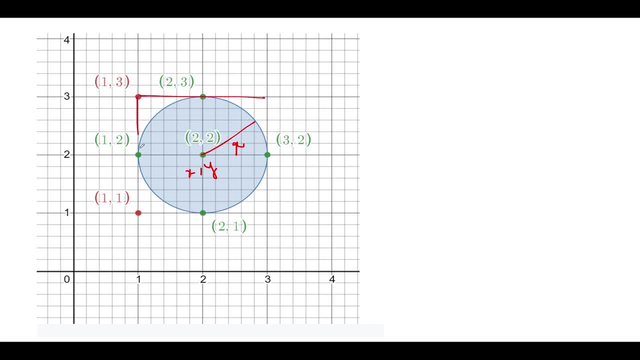 For that, let me just draw a rectangle around this circle. and let's draw this rectangle So we are sure that x, comma, y and the values of r will be in integer format. This was specified in the question, And what would be the coordinate system of this rectangle? So this point would be: 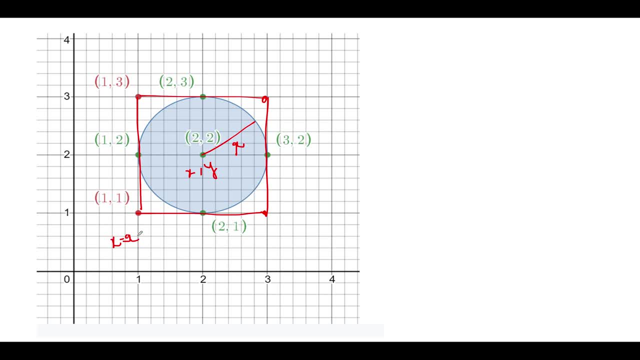 nothing but x minus r, comma y minus r. This point would be equal to the coordinates of this point, would be equal to x plus r. Now what we can do: We can simply iterate over all the coordinates that lie within this rectangle, All the integer coordinates, and we can simply use the mathematical formula. 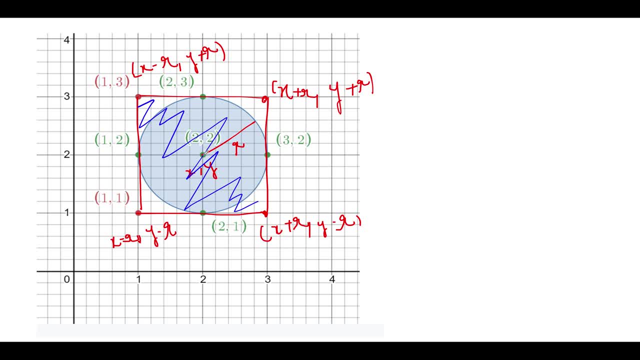 to identify the distance between a given coordinate and the center of the circle. If that distance is less than r, that means it lies inside the circle. If it is beyond r, that means it lies outside the circle. And while drawing this rectangle around the circle, we have 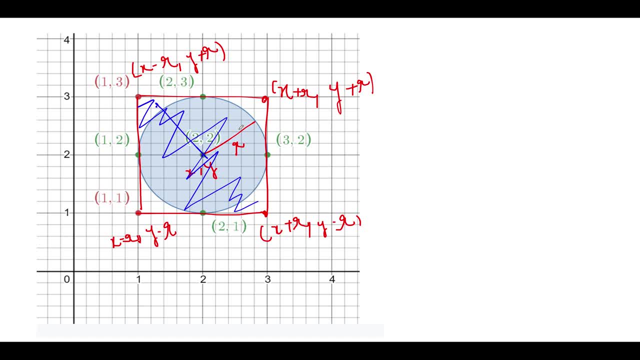 identified all the integer coordinates. So let's quickly shoot for the coding section and I'll explain everything there. But just remember that we draw a circle so as to identify all the set of integer coordinates. Then we apply the formula for finding out the distance between a coordinate and the center of the 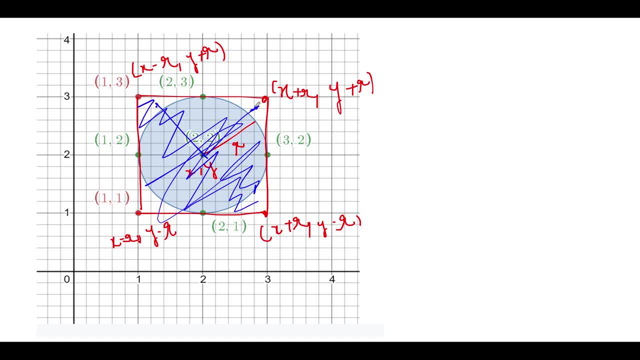 circle, And if, in case, that distance turns out to be greater than r, that means it lies outside the circle. If it is equal to r, that means it lies on the circle, And if it is less than r, then it lies inside the circle. So let's shoot at the coding section and 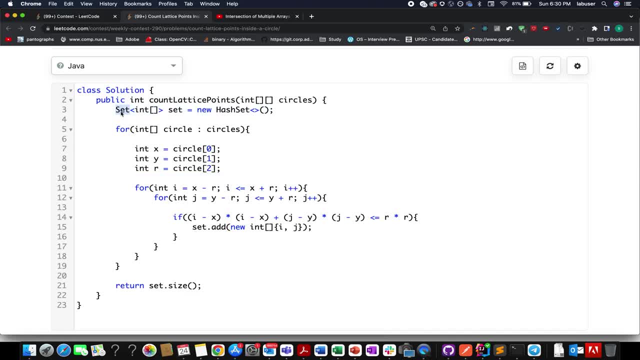 conclude the approach Here. I have created a set. I'll talk about the data structure of the set, why it is being used and its generic type, But let's shoot for the iteration that I want to focus on. I iterate over all the circles. I extract the center of the circle x coordinate. I extract: 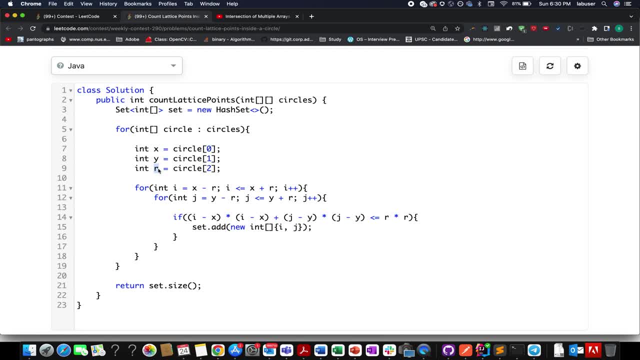 the center of the circle- y coordinate and the radius of the circle. And then I go and identify all the integer coordinates that lie in that rectangle zone. What is that rectangle zone? It starts from the x coordinate. It starts from the x coordinate. It starts from: 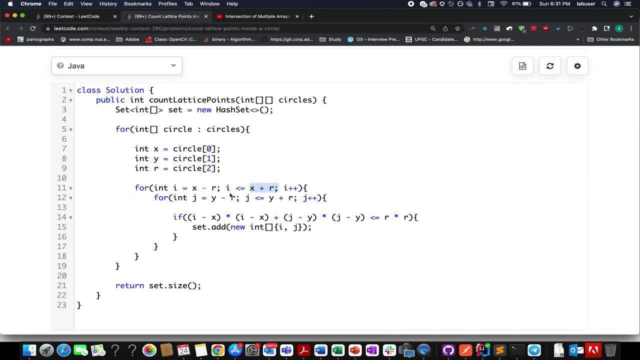 x minus r goes up till x plus r. The y coordinate starts from y minus r goes up till y plus r. And then I go ahead and identify the distance of that i and j coordinate that I have identified on that rectangle with respect to the center of the circle And if that distance happens, 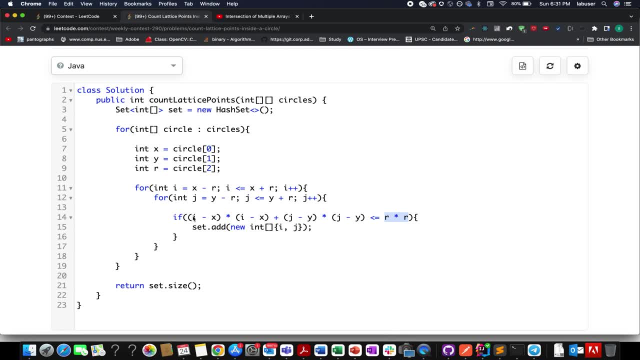 to be less than or equal to r square. that means the i and j point lies inside or on the circle. If it does, then I add it to the set, Otherwise I skip it up. And this set will store the coordinates of x comma y, so as to avoid overlapping situations. For example, a coordinate was: 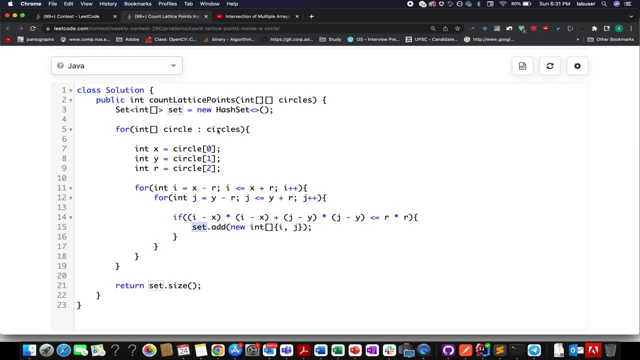 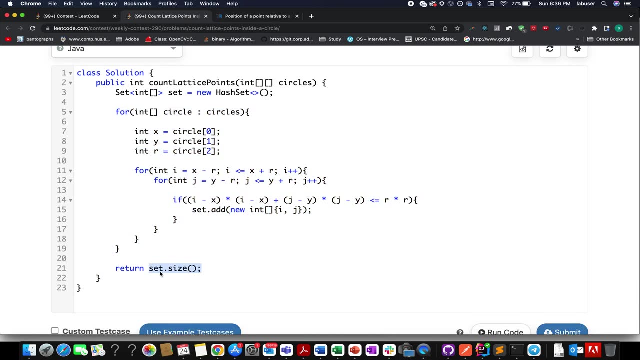 added into your answer by virtue of one particular circle and then it again got added by virtue of another circle. Therefore, we don't want to add overlapping answers onto it. Therefore, we have used set here. Once I'm out of this loop, I simply return its size It gives us. 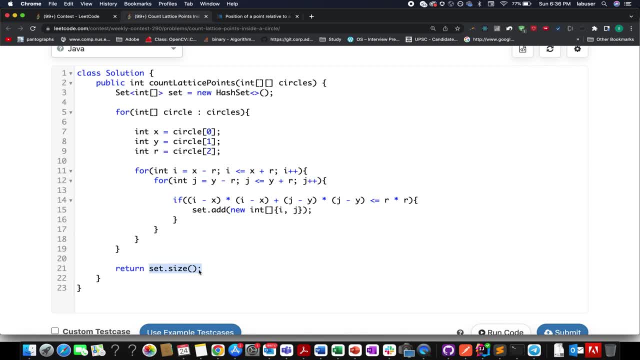 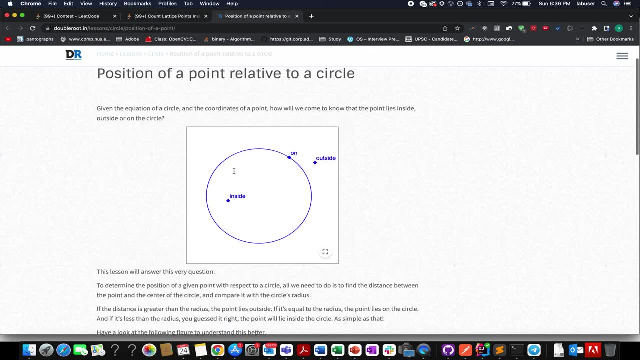 the number of lattice points that exist on any of the circle. And if you're confused about this formula, how to derive this up. I am attaching a link to a very good article wherein they clearly show how to identify a point, whether it's inside the circle, whether 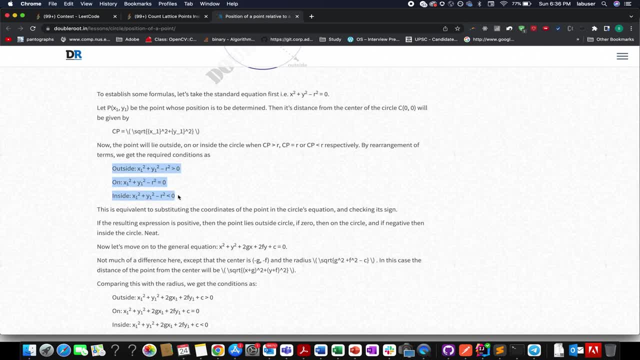 it's on or whether it's outside. This is a formula that they have specified. I have exactly used the same formula Here. x one and y one signify the distance rather than coordinate. And in case the distance of x plus x square plus y square is greater than r square, then x square plus y square is greater than r square. This is the exact same structure And I'm going to define a number of lattice points that exist on any of the circle. And, if you are confused about this formula, how to derive this up, I'm attaching a link to a very good article. 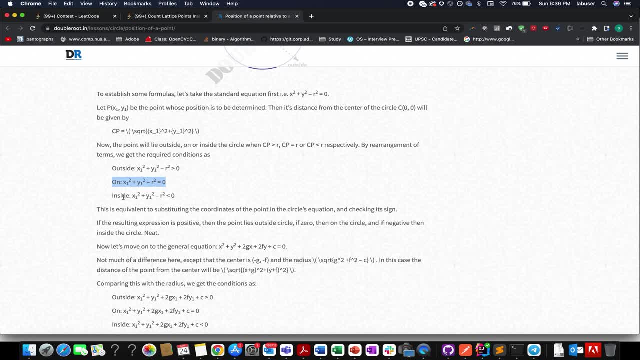 square, that means it lies outside. if it is equal, that means it lies on the circle. if it is less, that means it's like inside the circle. so i've used these two formulas over here and remember x1 and y1 here have different meaning, rather what we have specified over here, so that with this let's